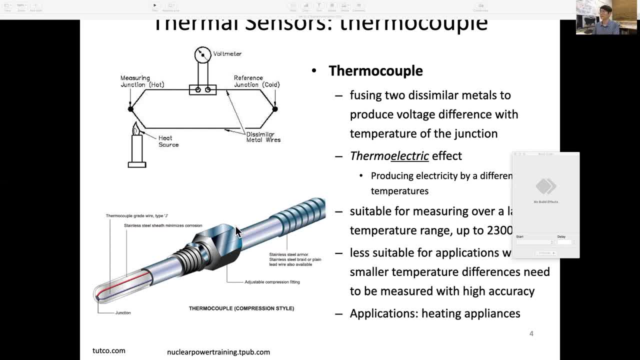 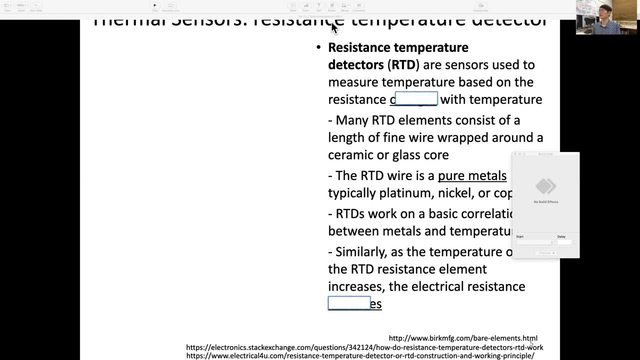 that this thermocouple has been used. And the second is: I want to introduce this so called RTD element, which is Resistance Temperature Detector. So these RTD are sensors used to measure temperature based on resistance changes with temperature. And how does this RTD, or Resistance Temperature Detector, looks? It's a very fine wires wrapping. 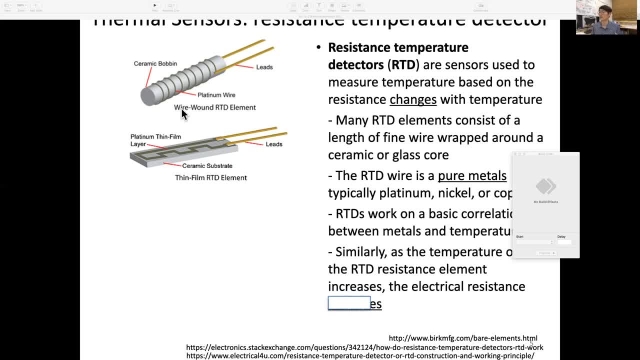 around a ceramic or glass core. So here's the two examples, with this ceramic very fine wires wrapping around. So when the temperature changes and these substrate thermal expansion will affect the wire, Then it can be used for the temperature changes sensor. So this one is a platinum thin film. 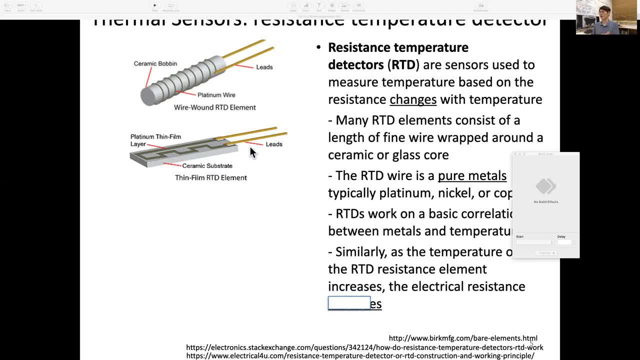 layer with on the ceramic substrate and there's a lid. So this RTD or Resistance, Temperature Detector wire is usually a pure metals, typically platinum, nickel or copper. So so this resistive, resistive, resistive, resistive. 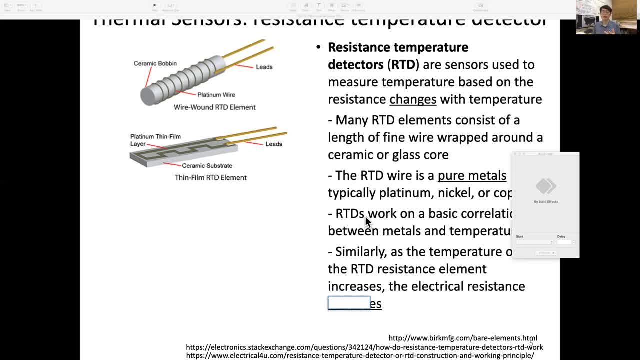 resistive, resistance, temperature detectors working on a basic correlation between these metals and the temperature, And so it looks almost like this ceramic and this is a thin film, And so let's see the this actual data. So when the temperature rises, thinking about this, the relative resistance. 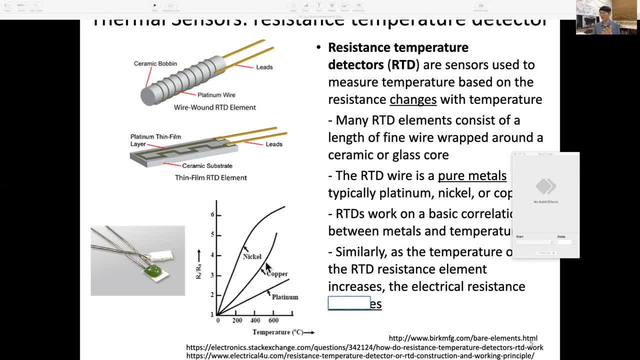 also rises with different platinum, cotton, copper and nickel. So as the temperature element increases, the electrical resistance also increases. So this is my theory on this. so that ceramic or glass substrate were thermal expand when the temperature rises- And this is a very thin wire, will also elongate, So the diameter 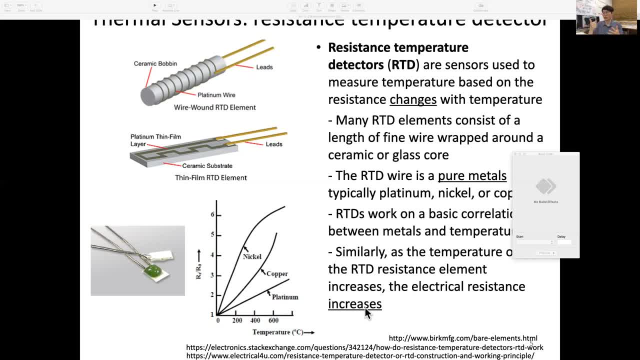 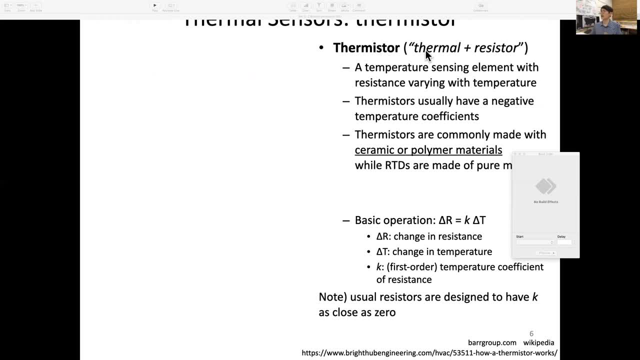 or cross-section goes down, so the resistance will increase The energy distribution in this territory. for this thisunts are somewhat a bit more pressureños으로 resistance will goes up. The third one I want to discuss is thermistor. So thermistor means a thermal plus resistors ester, So that's a temperature. 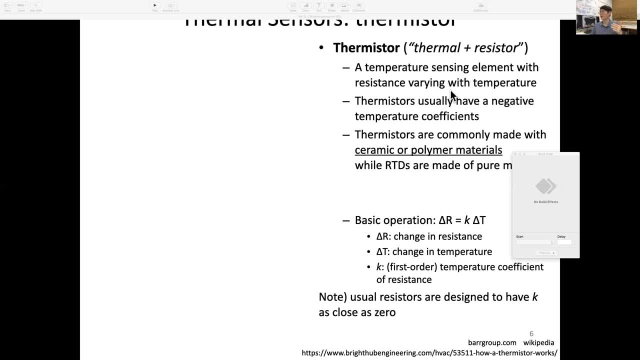 sensing element with the resistance varying with temperature, And usually it is a little different from RTD resistance temperature detector that this has a negative temperature coefficient And because- and that's because- it's made with a ceramic or polymeric polymer materials, not a pure metals like RTDs. 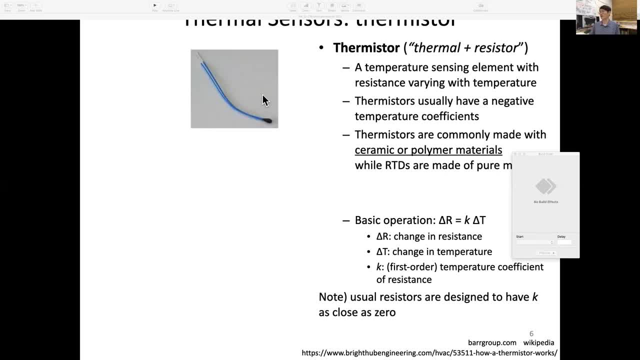 So it looks almost like it's very simple and how we operate them. I give you an example here, So that these are thermistor and we have a resistance and this is a op amp with a follower and to measure the voltage to analog, to digital conversion converter as an input. So this needs a 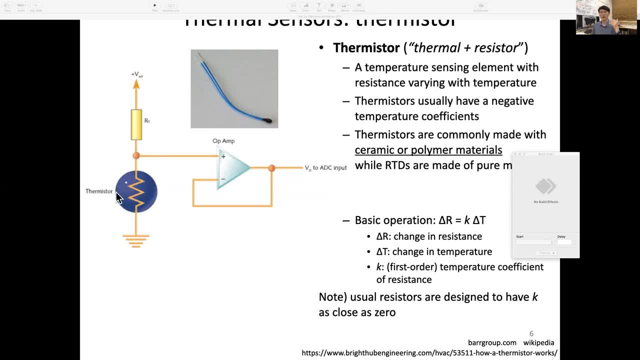 circuitry, that you see this thermistor, when their temperature changes, this resistance changes And you see, this is a voltage reference and this RT and this thermistor, resistance, is a voltage divider and that you measure it with this voltage follower. So the basic operation is resistance. 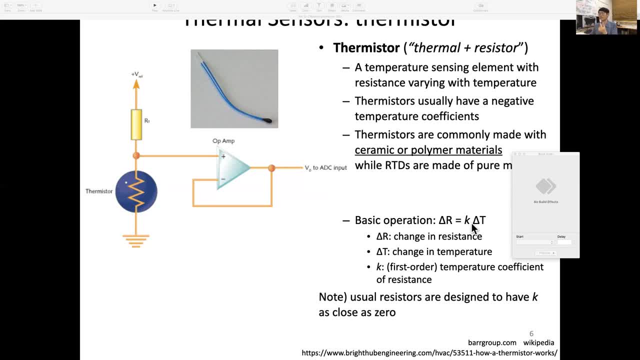 changing is supposed to be related to temperature change, with a constant as a first order. So look at these data, compare. compared with RTD versus thermistor, you see much large resistance changes you can see. So it has a higher gain or sensitivity, and and also the slope is opposite. So then Then it is when 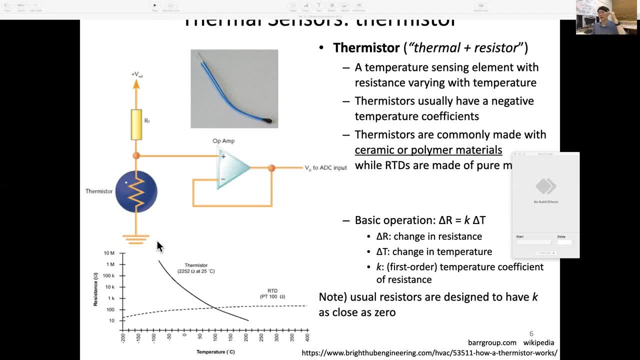 temperature rises, this thermistors resistance actually goes down. And further, note that typical resistance resistors, which you don't want it, change it to resistance over time. So these are designed to have K as close to zero thesis. So these are designed to have k close to zero, but in thermal sensors or thermisters. 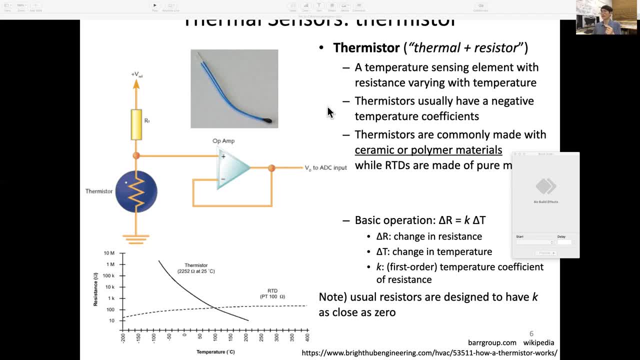 So, while it cannot be converted back into thermal talking, that is, the gas temperature confronts with a constant density of the indicates reading number. So, whether it is πο, vibrance number, omission limit is feet up. temperature: various high frequencies use for temperature perspective data and this is 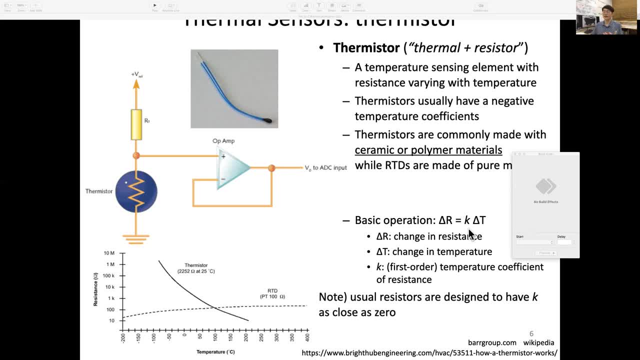 смотрите. So the norm is: enter and show a temperature and if tempo. mostly you want the K as big so that it can be more sensitive. So to describe this, people have developed this empirical formula too, and you can at a certain